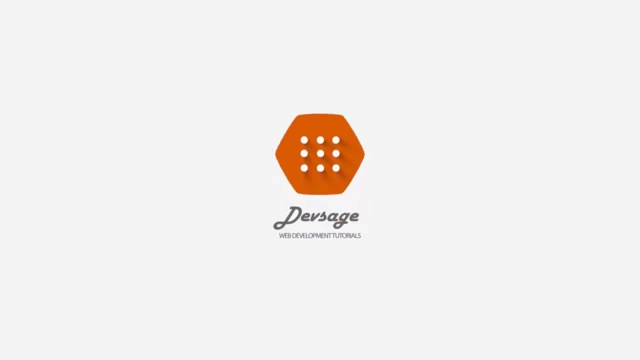 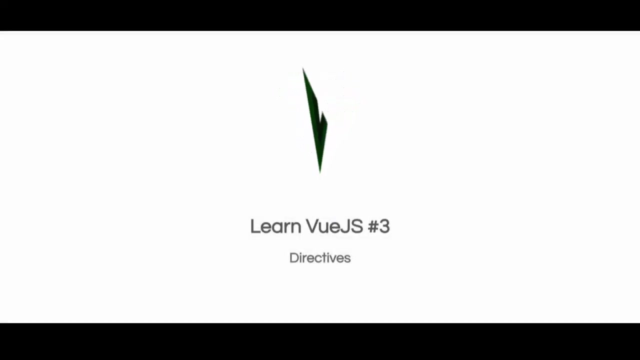 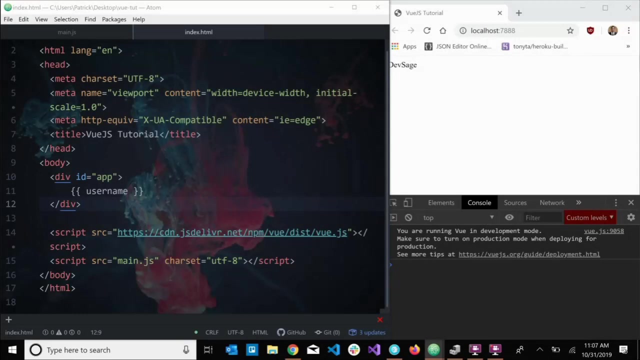 What is up, people DevSage here, and in this video I'm going to be teaching you about Vue directives. In the last video we went over the basics of the Vue instance. In this video we're going to expand a little and talk about Vue directives, But first I want to quickly go over 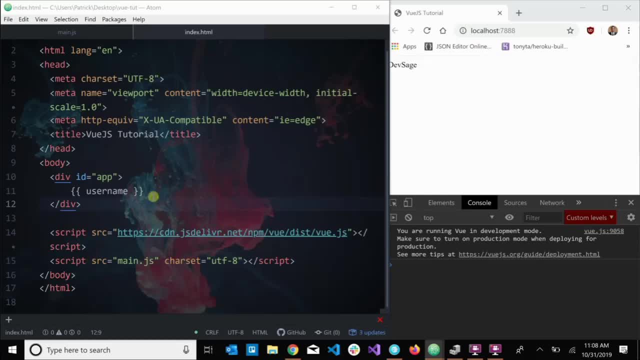 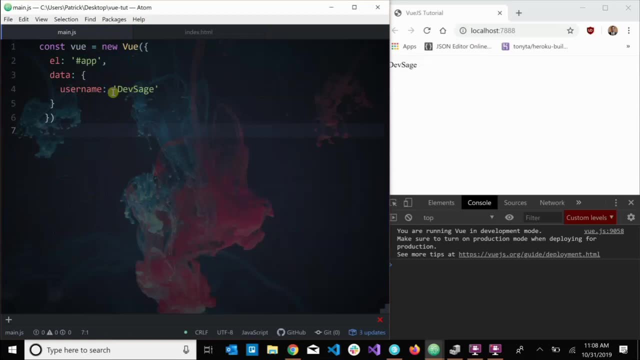 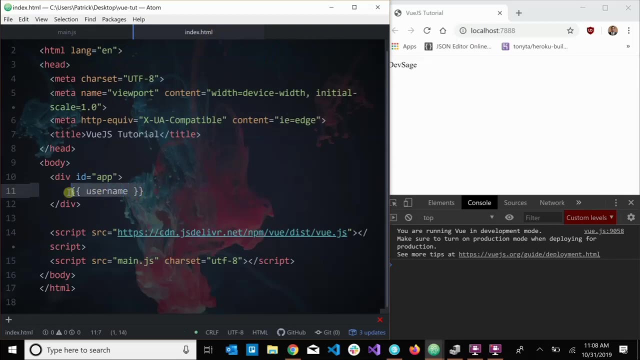 one thing we talked about in the last video, which is this: Remember how we defined username here in our component and we were able to inject that username into our HTML using these double curly braces. Well, this username here, this is just a regular javascript expression. I mean so whenever. 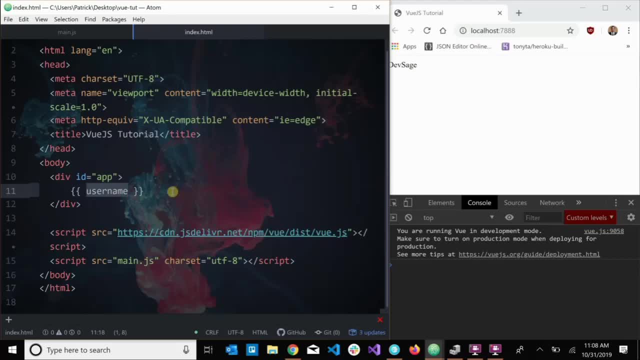 you want to evaluate actual javascript in your HTML, you just wrap that javascript with two sets of curly braces and Vue will automatically determine: hey, this is javascript. There is a limit to what you can put in here, though. These curly braces can only accept one expression at a time, So I can you know. you see that we can inject variables from. 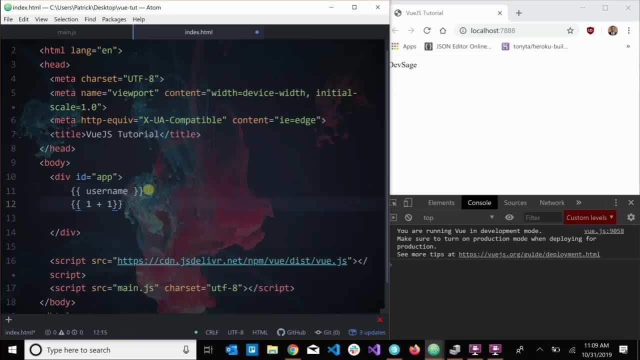 our component, but we can also just evaluate regular javascript. I can put one plus one and that will evaluate to two over here, as you can see, I could do ternary operators. I can do one less than two. Return true, else false. Now return true. as you can see, There are limits to what you can do, So I can't do this. I. 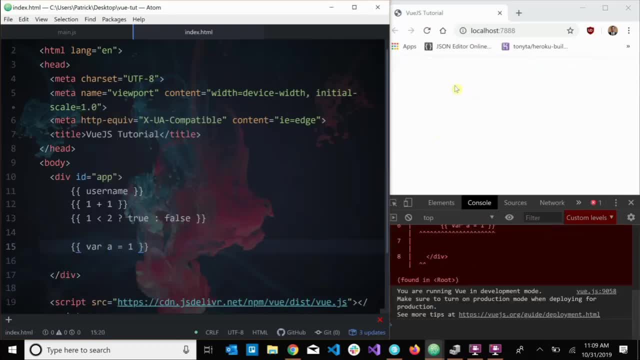 can't do var a equals one. This is a statement. You see how it breaks the whole thing. Everything disappeared. and I have an error in the console. Vue can't evaluate statements, They can only take in expressions, So this is bad. Comment that out. Likewise, I can't do flow control, so 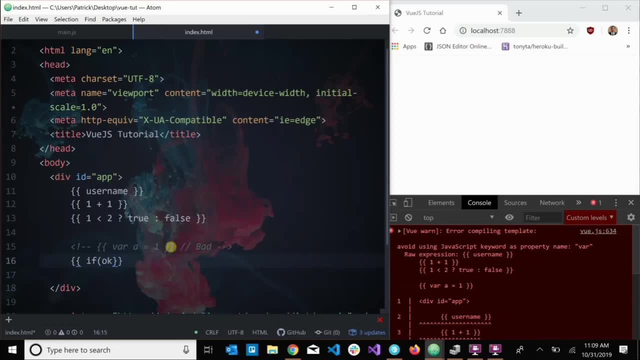 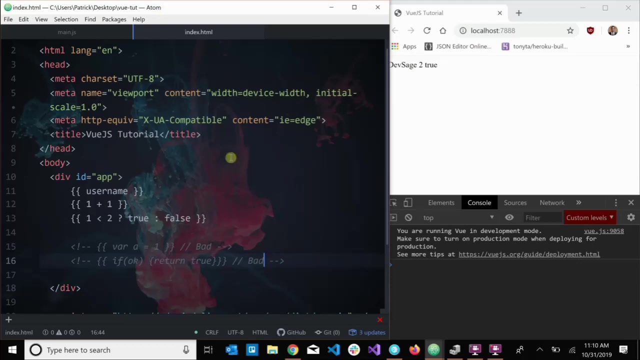 I can't put if okay, return true, I can't do this either. This is bad. It's bad, But yeah. So, yeah, yeah, there are limitations. you can only put expressions. you can only put one expression at a time. but you know, if you have any complex logic, you really don't. 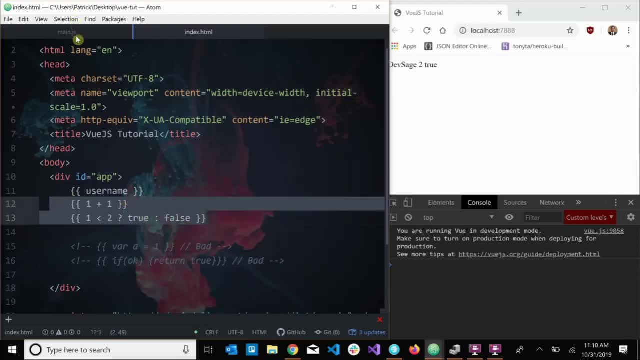 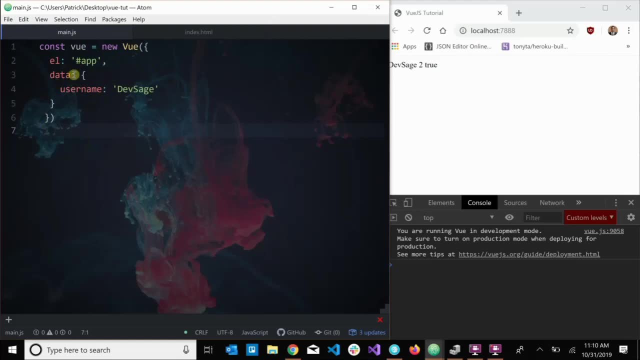 want to be putting that here on the front end. if you have any complex logic, really that logic is going to be handled by view instances on the back end here, or view components when we go over those in a later video. but yeah, that's just a little bit about expressions really fast, but now we can actually get into view. 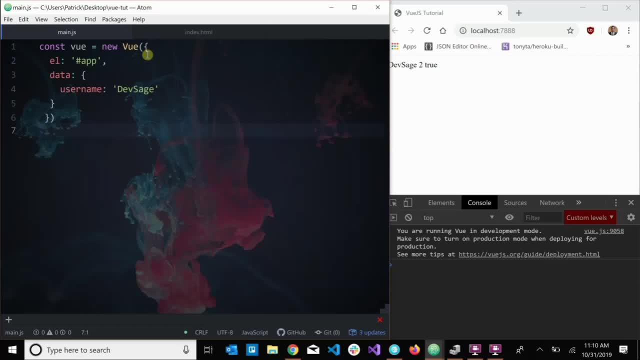 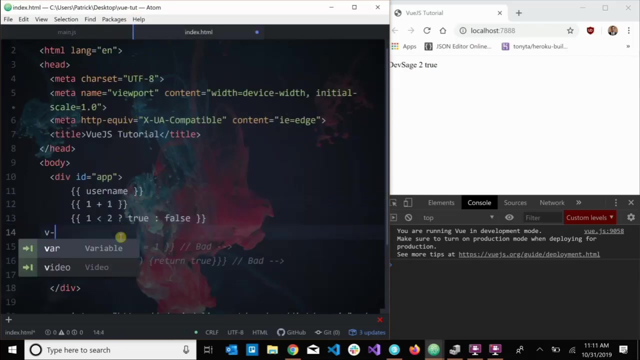 directives. so what is a directive? a directive is a special attribute that you can use on HTML elements, kind of like class or ID or style, except view has its own set of attributes, and they all start with the V dash prefix. so so what a directive does? it applies certain effects to the Dom when its 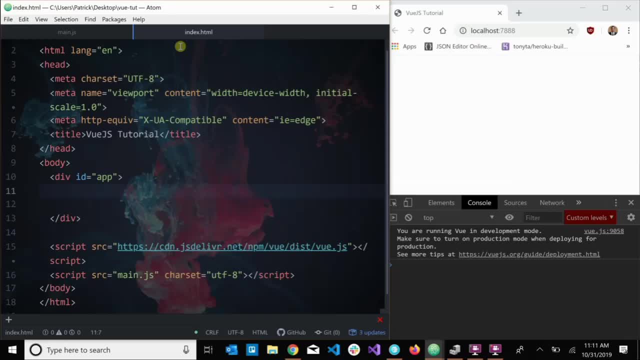 value changes. so some examples of some directors are VHTML, for example. I'll actually do an example here. so let's say I have a span and then let's say I want to, I want to use VHTML. what VHTML does is it takes in a JavaScript expression. more than likely, this expression is going to be a 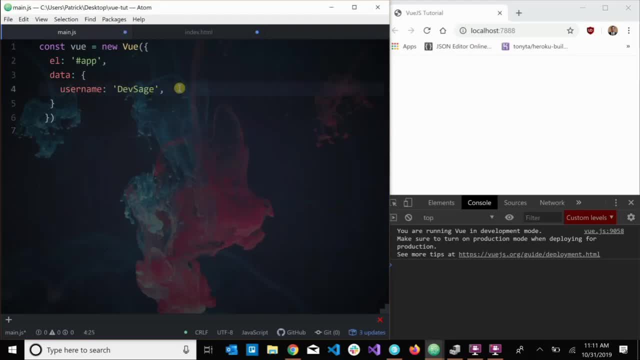 variable coming from your data. what you can do is you can say: let's say, I want to name this HTML and I want to inject actual HTML code into my, into my HTML file, my indexhtml. I can say: let's let's just say: DevSageTutorialscom. 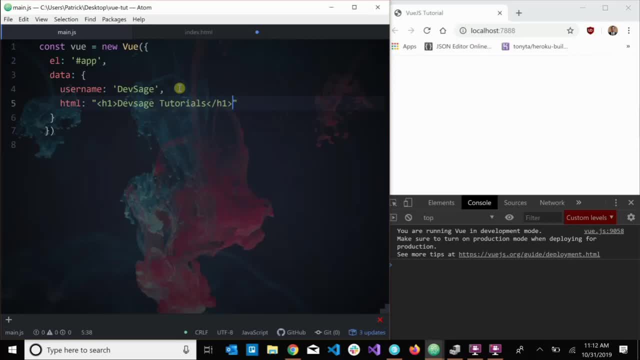 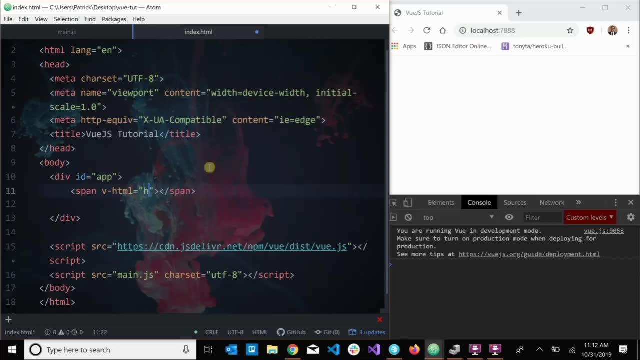 boom. so now i have a property on my instance called html and i can inject that into my span here and, as you can see, dev stage tutorials. well, you might say: well, dev, why don't you just do something like this? why don't you just put html? well, that's because this is strictly 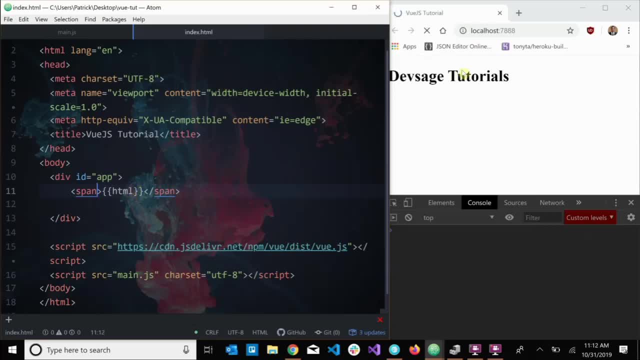 text interpolation. so this is going to take that exact string that i typed in and it's going to render that just like how it is in the component, whereas if you did a vhtml, that's going to say, okay, i'm going to evaluate this just like html. 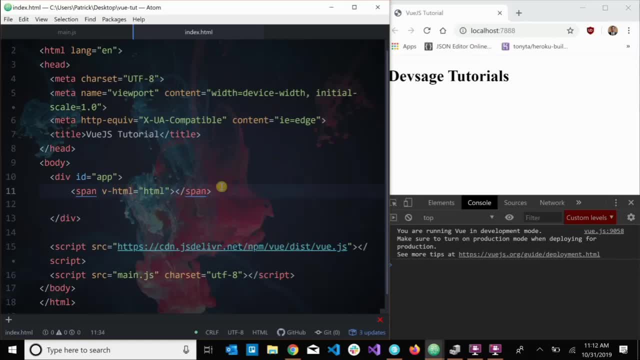 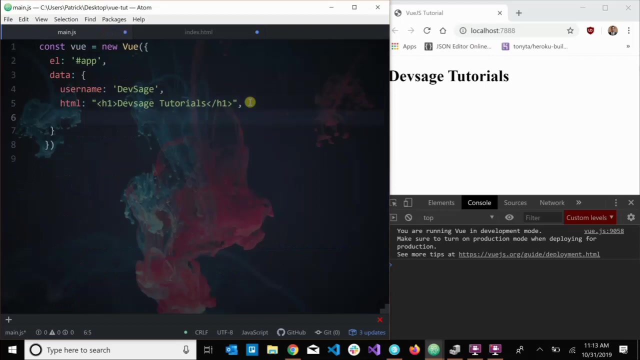 so another uh directive is the um if, the if directive. basically, this just takes that string and it's going to render that just like how it is in. the component just controls whether or not an element is displayed on the screen based off of some condition. so let's say I go back and I added a new property on my data. 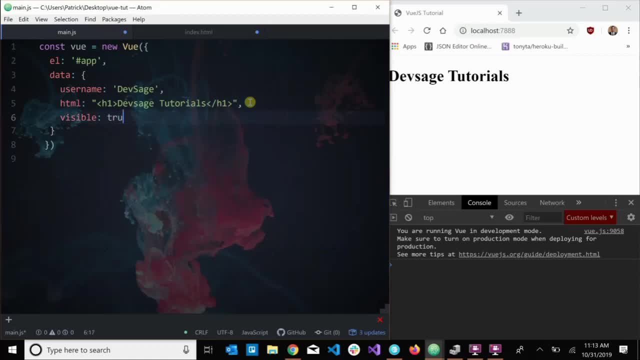 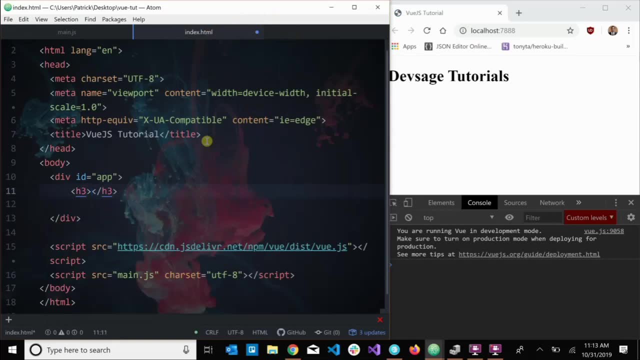 called visible and I set it to true. and I go over here and let's say I have h3 and this h3 is going to have something random. I'm just going to put random. I can control whether or not I want to see this by putting the if, and then this likewise takes in an expression. I could just put false in here. 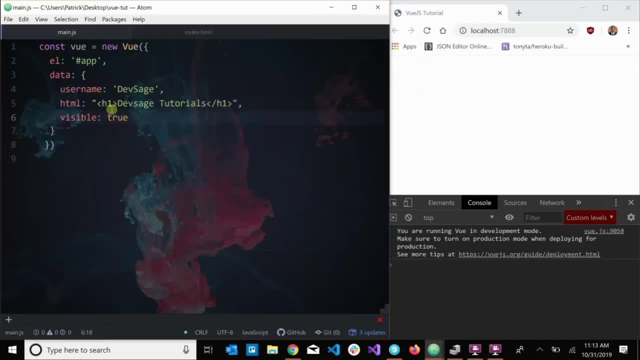 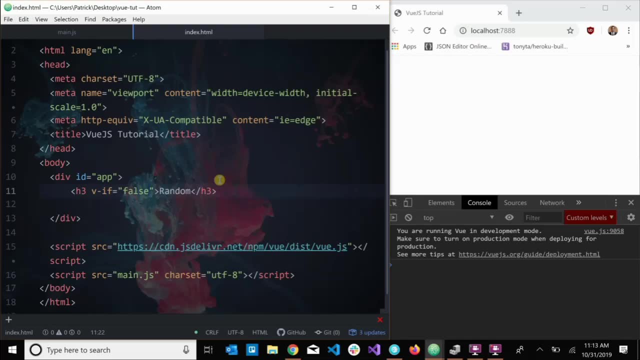 if I wanted to and it wouldn't display. but we're actually going to be using that visible data from our component, I mean our instance. I keep saying component- we get to components later- but these are just instances for now. but you I can, I can put that in here and right now it's set to true, but I can easily go. 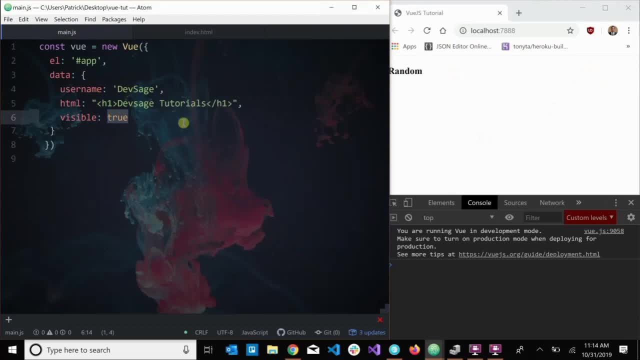 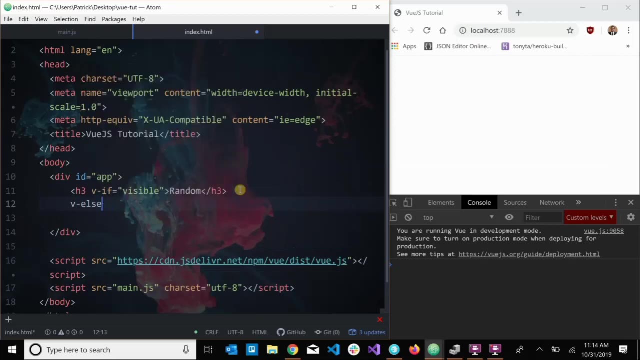 in on the back end and say: well, not back end, but I can easily go in in my main js file changes to false and it wouldn't display we also have the else if and we also have the else, and you can probably imagine what those do. basically, you can just string more conditions on onto your if statement and then display different items based off of where the conditions. 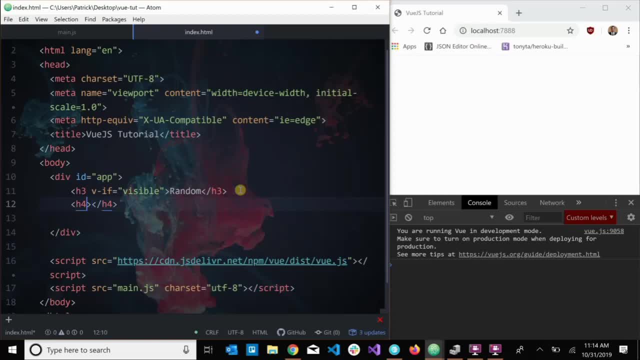 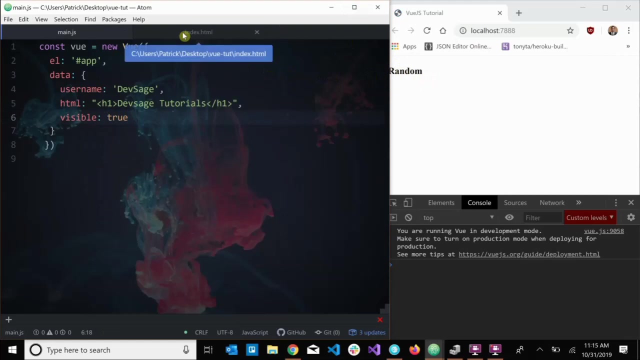 are false or not. so I can put h4 v, else not random, and then one of these would display but not the other. so since visible is set to false, right now not random is displaying. but if i set it to true, random would display and not random would be off the screen. 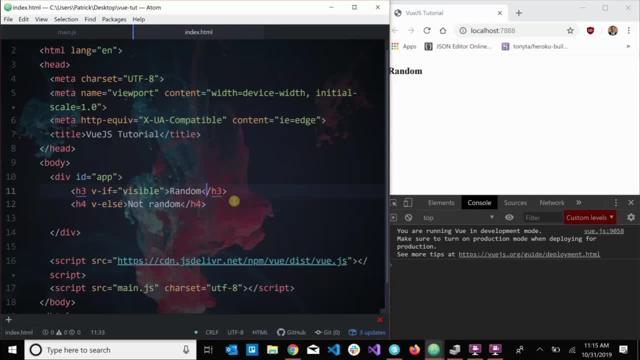 so this works for single elements. what if i want to do? what if i want to this? what if i want mult to display multiple elements? what if i want to control multiple elements at the same time, so i can wrap these? let's say i have um. let's just say i have um, an h3 called one, h3 with two, and i. 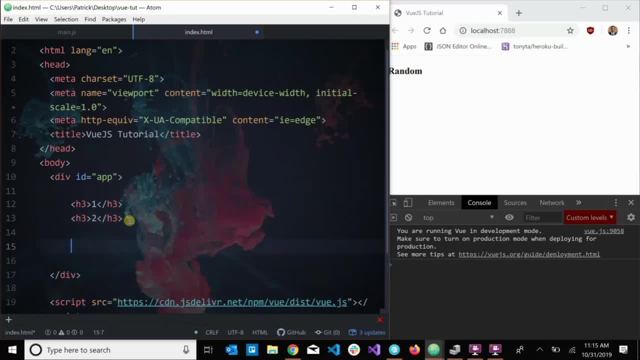 want to either display both of these, or i have an h3 with three, an h3 or four. so let's say i want to display either both of these or both of these. well, i can't put ifs on both of these, right? i mean, i guess i i could, but what if i had a hundred elements? i mean, 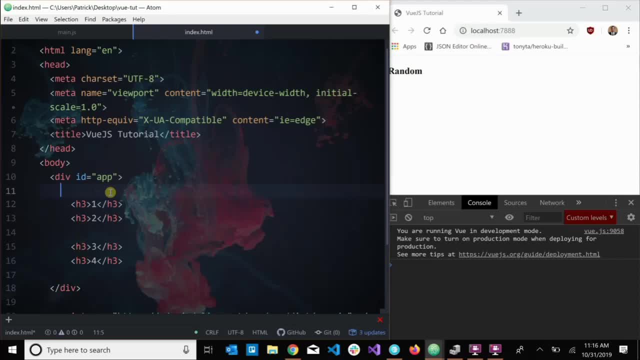 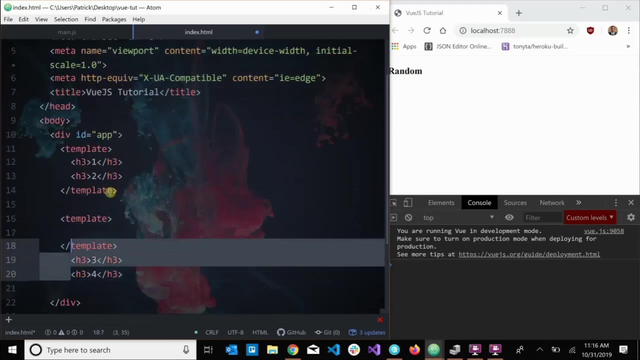 i would have to put ifs on all of those. well, no, i don't. actually. i can just use the template tag and i can wrap this template. i can wrap my- uh, my html with templates and i can put my if statements on my template: the if visible. 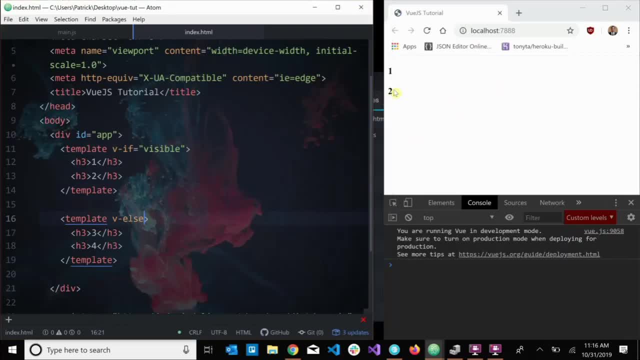 the else. so right now i just have one and two, because visible is set to true and three and four are hidden. what does template do? template actually doesn't render any html on the screen at all. it's specific, i believe it's specific to view. it doesn't actually render, or? 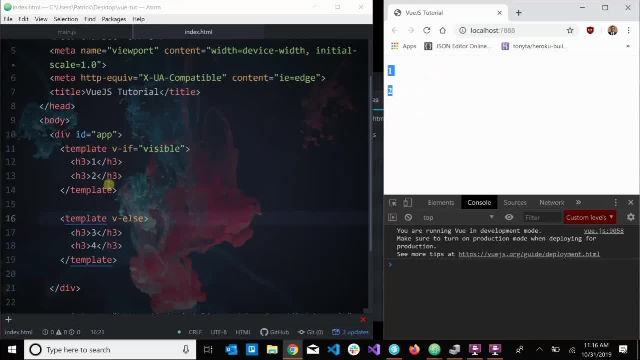 add anything. this is strictly for con uh just creating blocks to tell view. hey, this information belongs to each other. i mean these, this group of information uh just needs to be grouped together. there's nothing special about the html it outputs or anything, so that's a little bit about directives themselves. 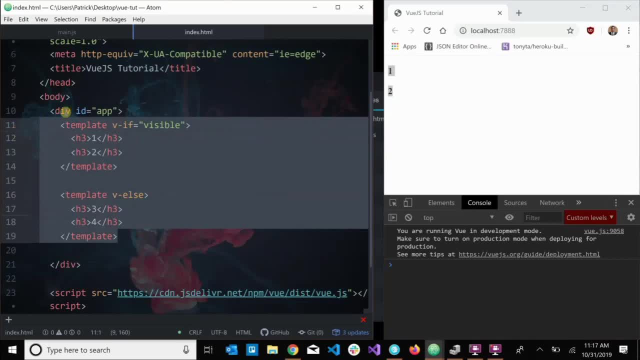 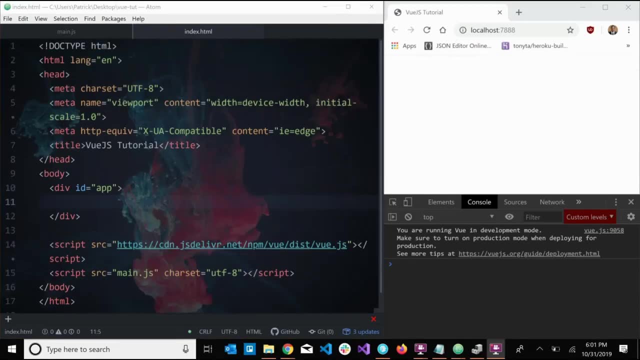 directives can actually take in arguments to further control how they behave. so an example of a directive that can accept an argument is the v bind directive. so what the v bind directive does is it takes a real html attribute like class or id or style, and it binds it to some value or some variable. um, let me show you what i mean. so let's say i have 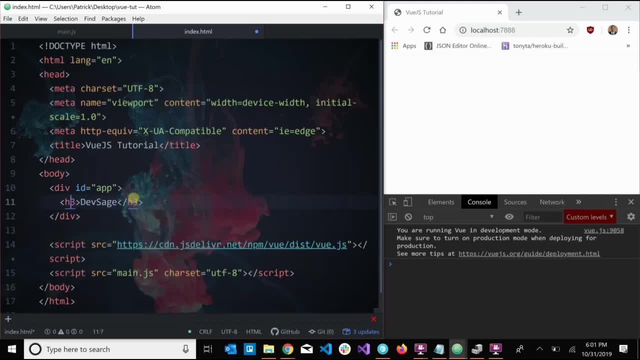 an h3 dev sage and i want to let's, let's say a v bind and then this colon tells: this tells view. okay, i'm passing an argument to this directive. in this case, the v bind directive takes in an html attribute for an argument, so i'm going to just give it a class and i'm going to say equals. 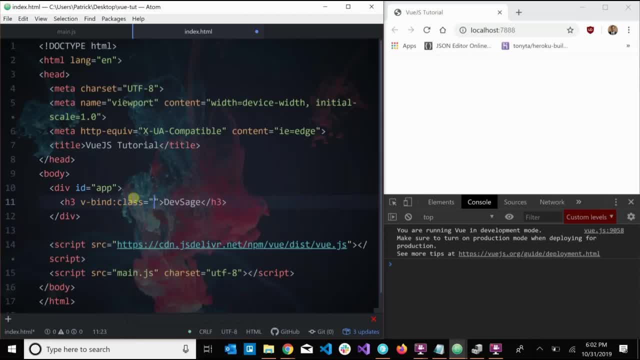 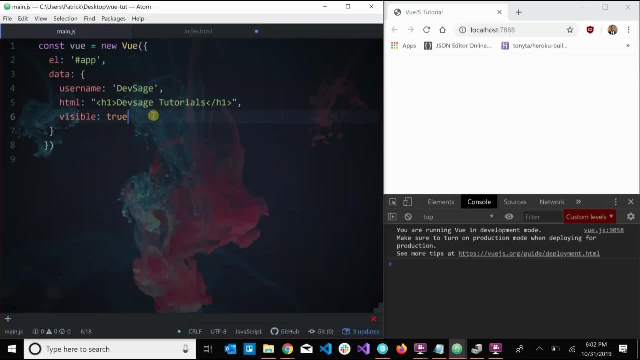 and here i pass in some javascript expression that evaluates to something. in this case let's go back to our view instance and let's make a, a new property here, and we're going to inject that and use that as our class. so i'm going to just name this property red and then i'm going to 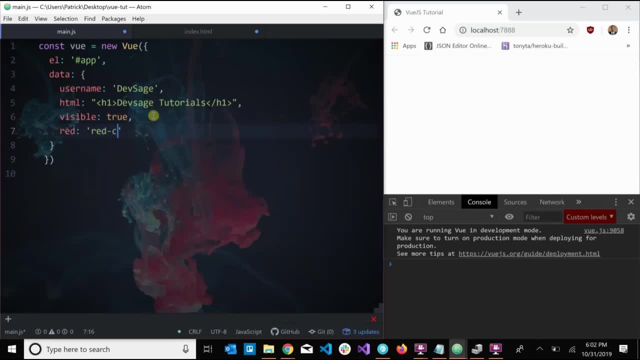 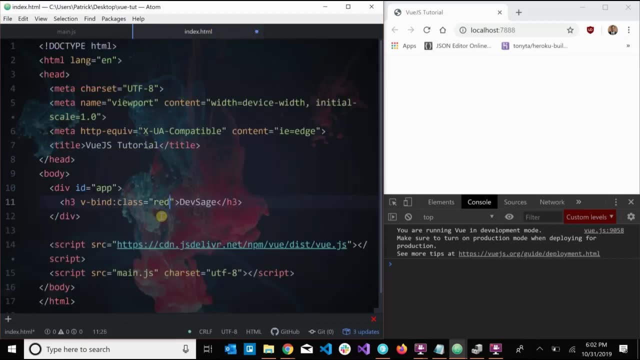 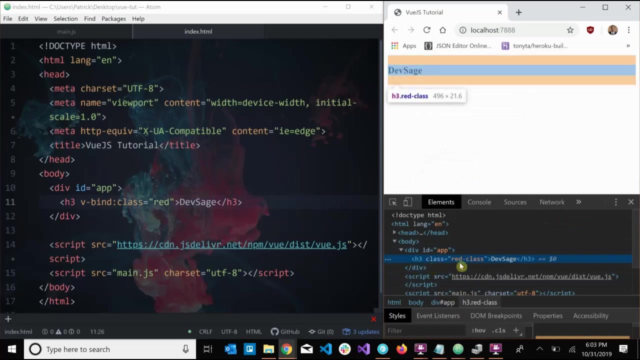 give it the value of red class. let's save that. and now we can take red here and pass this in, because this is just a, it's just the javascript expression. it's going to be evaluated. so let's save that, okay, and let's actually inspect this. and, as you can see down here, h3 class, red class. 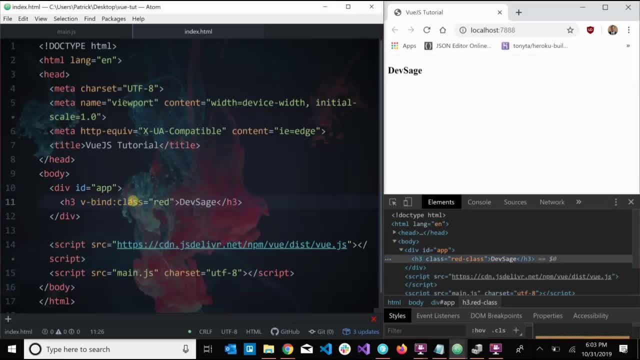 so yeah, that's how the v bind argument works and you can pass in anything here. you can pass in style or id, height, width, whatever. uh, the v bind argument, the v bind directive, takes in any valid html attribute for an argument. okay, so that's v bind. uh, one other directive that's pretty popular that takes in an argument. 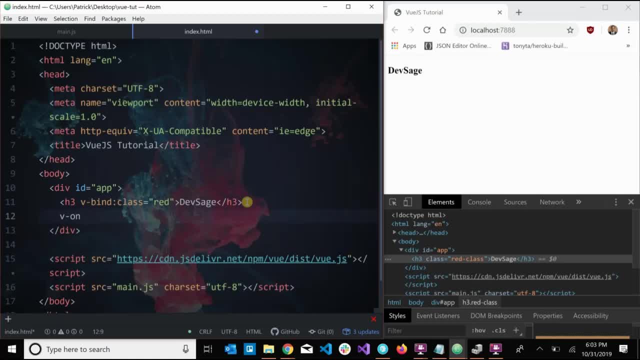 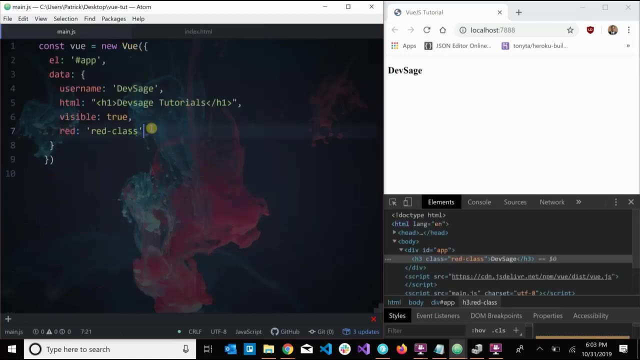 is the the on attribute, so v on basically just acts like an event listener. so let us say we have um, let's. let's go back to our view instance and we're going to build a counter. so i'm going to add a property called count, i'm going to initialize it to be zero and then i'm going to come over here. 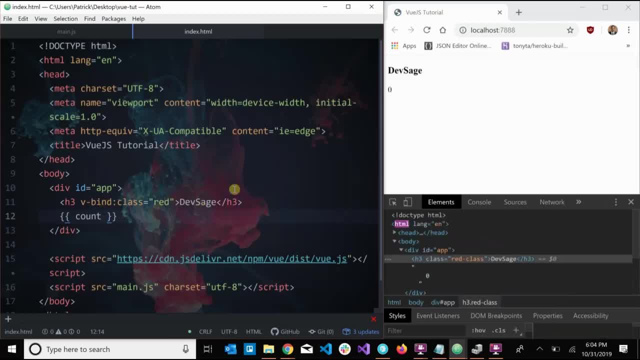 and i'm going to inject count into our view and we have zero and let's say we want to have a button down here, button uh, and every time we click our button we want to add one. so i'm going to name our button: add one. okay, so how do we do that? we can say v on and we're passing in an argument and we 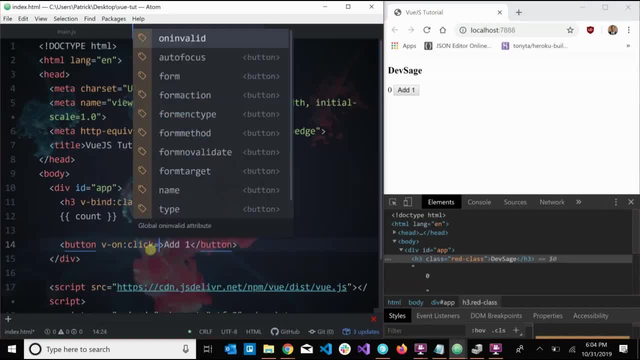 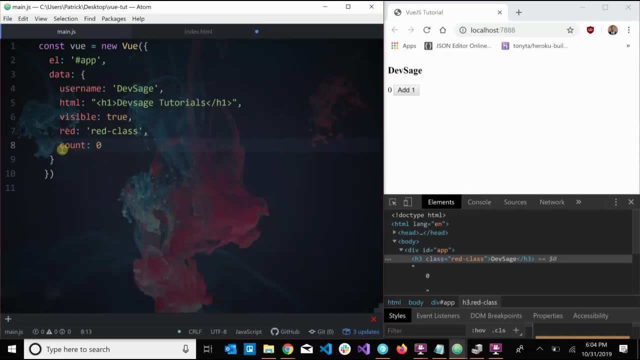 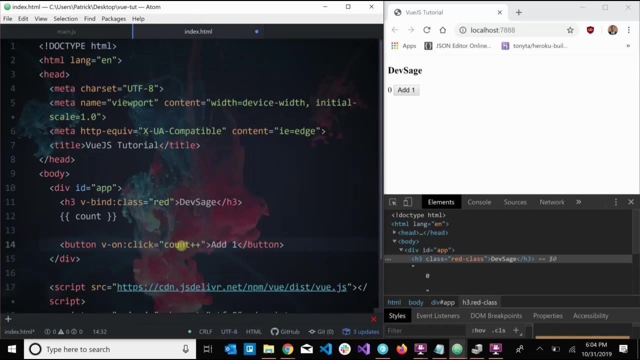 can pass in click and we set equals, some javascript expression. in this case we can actually increment count by one, so we can say count plus plus. because, remember, this is just javascript in here that's being evaluated, and let's save that and let's actually click our button. look at that: one, two, three, four, five and yeah, the v on. 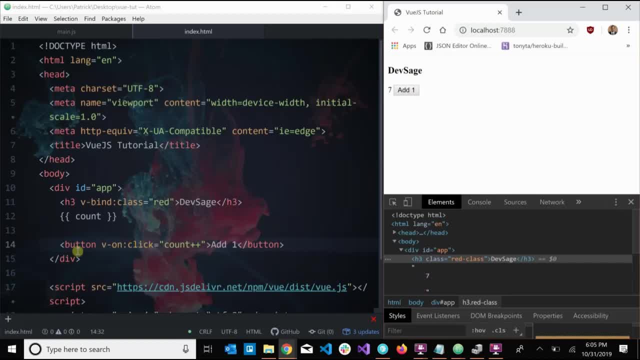 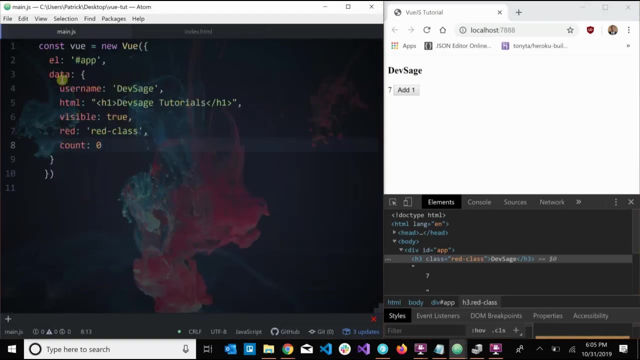 is binding the click event listener to this button and when it's clicked it evaluates whatever's in this uh, whatever uh expression is here. so in this case it's count plus plus. it updates count. the html says okay. well, view tells the html: okay, i've updated. so i need to update the view on the page, the view. 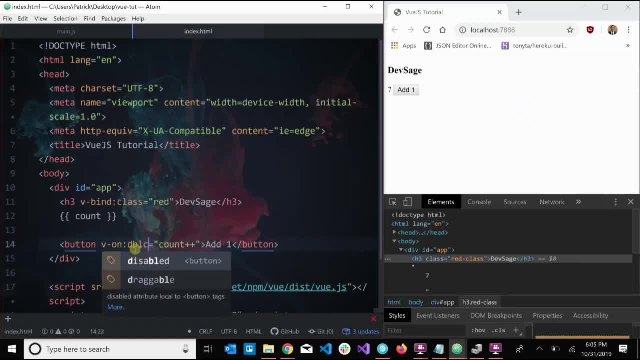 and i can pass in. you know, instead of click, we can pass in double click or hover or you know any, uh, any valid event. listener um one step further. directives can also have modifiers, which are special fixes, meaning that they come after the directive that indicate um that they should be bound in some. 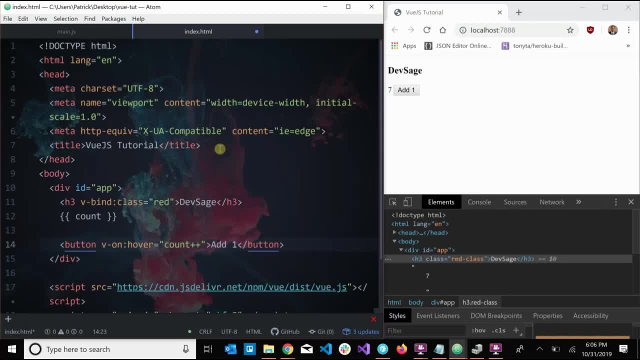 particular way. for example, let's- uh, let's go back up here, let's change this back to click. let's say i only want to um, let's say i only want to increment, increment, count. on the first click i can add an event modifier or directive modifier once by using dot once after my argument here: 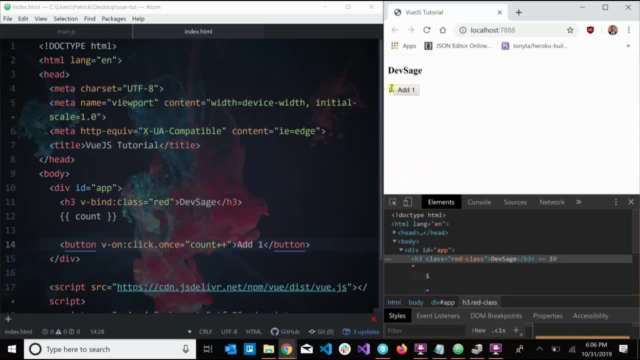 now what should happen is i should click on add one and it should increment the first time, but when i click on it again, it's not incrementing anymore. once is a directive modifier it, it, it tells the directive: okay, i want you to do this certain thing.